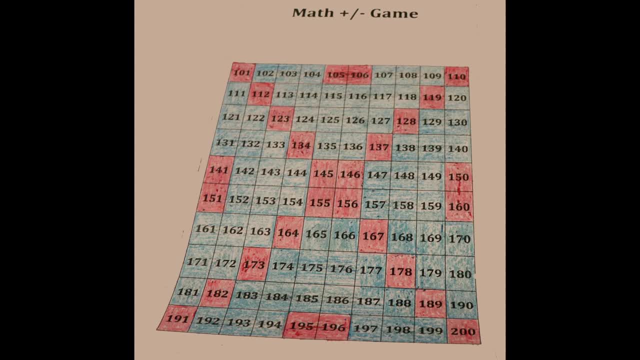 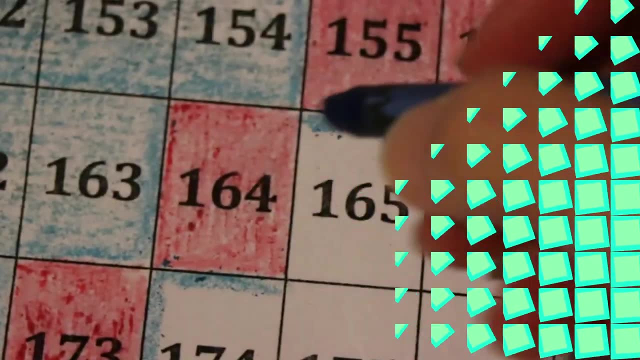 I played with the idea of mirrored patterns. So if you look at the top, bottom, left and right, they are all a piece of the same design, So it turned out to be a fun geometric X pattern. When you are doing your coloring, make sure that you pay close attention to the borders. 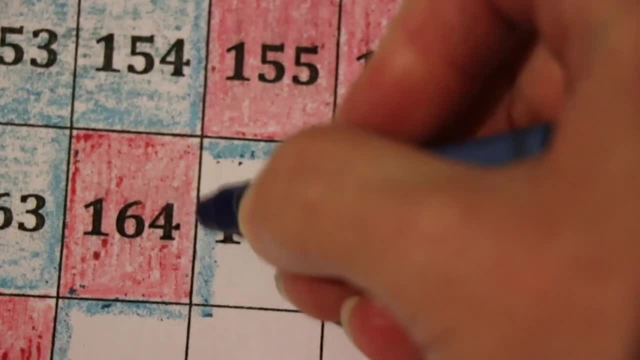 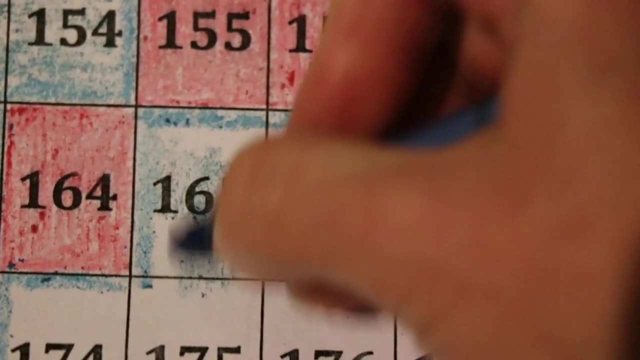 of each square. One thing that can help is to carefully and slowly make a thick line along the borders and then fill in the middle of the squares with more rapid coloring. This helps to make sure that you don't go over the lines or mix colors in other squares. 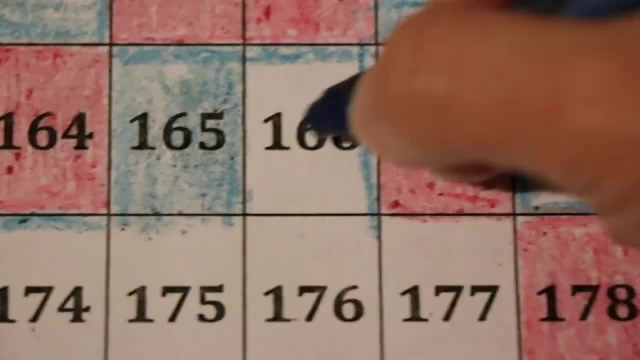 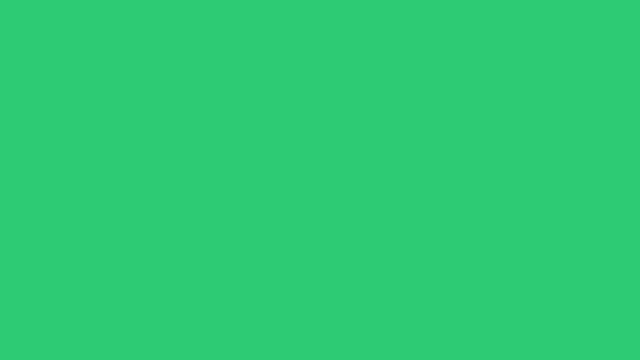 Remember you need to cover the entire board with color in all the squares. When you are finished, you will have a nice quilt design. After you have your entire board covered, it is time to make the color key At the top of the board. draw two small squares, one for each color that you used in your quilt. 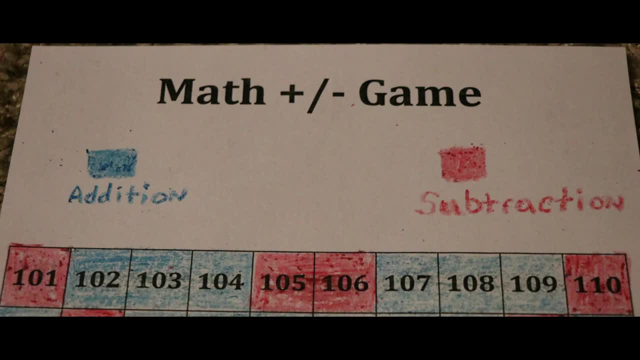 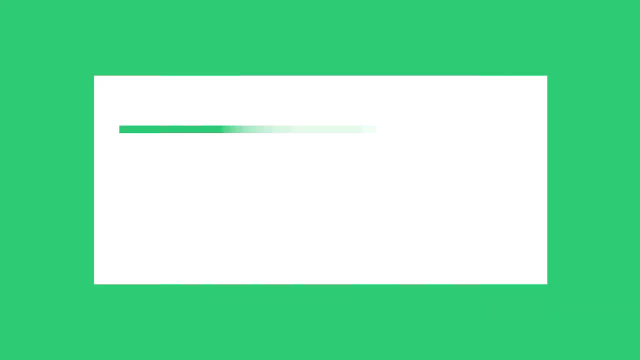 design Label. one of the squares addition and the other subtraction. This is what you will use to know where to move your markers when playing the game. Now it's time to play. Here are the rules. First, place the game board in the center of a table. The youngest player will go first. 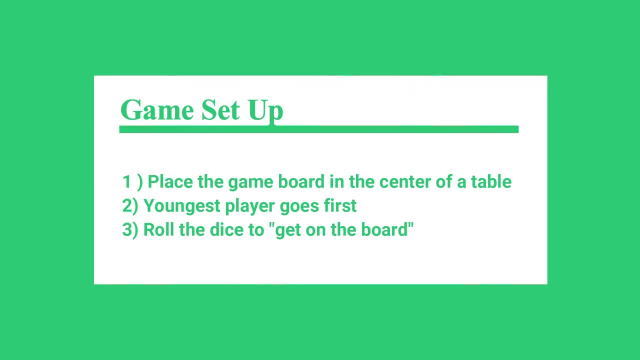 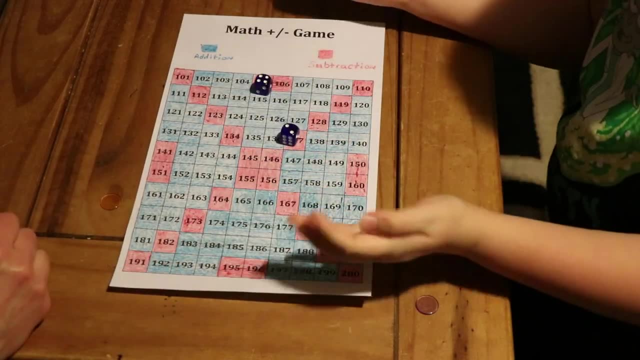 Roll the dice to get on the board. Every time you roll to get on the board you will be doing an addition problem. So, for example, here you will see the player one rolls a six. He puts his marker on 106.. Now it is the next player's turn. Roll the dice. 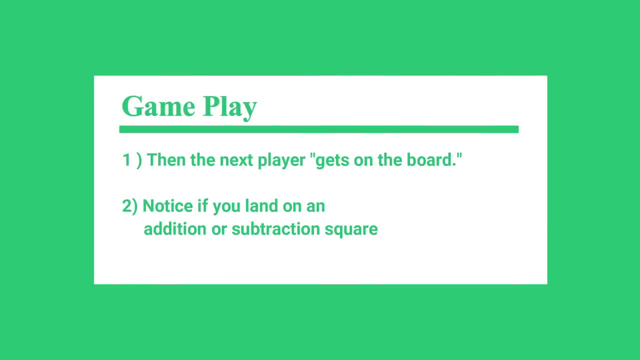 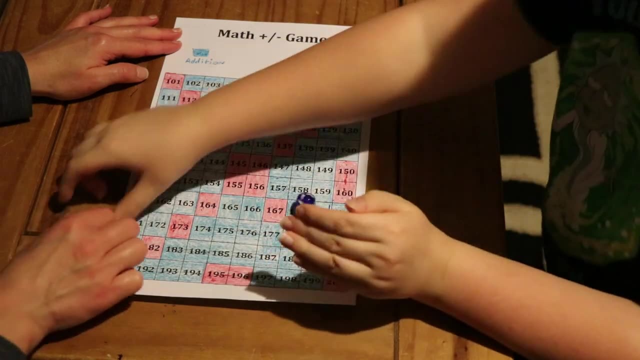 and get on the board the number of spaces rolled. Continue this until all players are on the board. Pay attention to which color you land on and if it is an addition or subtraction square. Now we are back to player one and they are going to roll the dice for their turn Here. 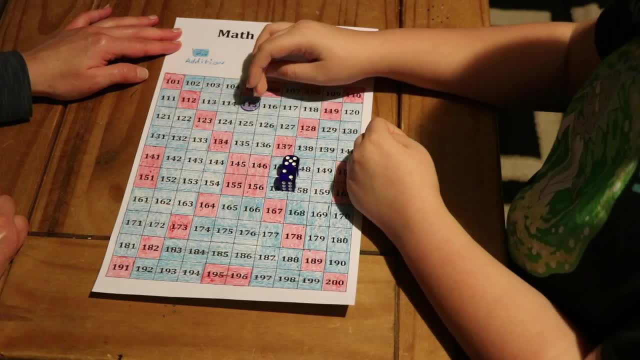 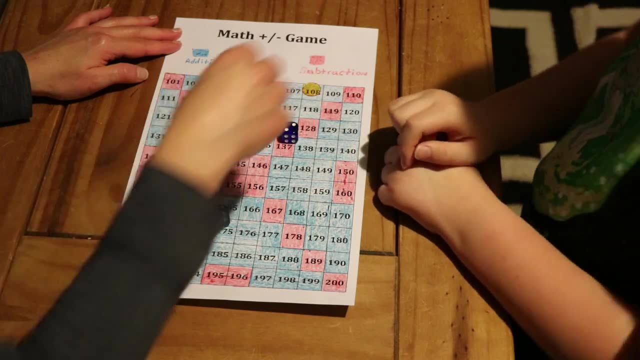 you can see that player one was on a blue 115 square. Blue is an addition square color in my board. Player one rolled a seven, so you will add 115 plus seven and end up on square 122.. If player one had been on a red square which? 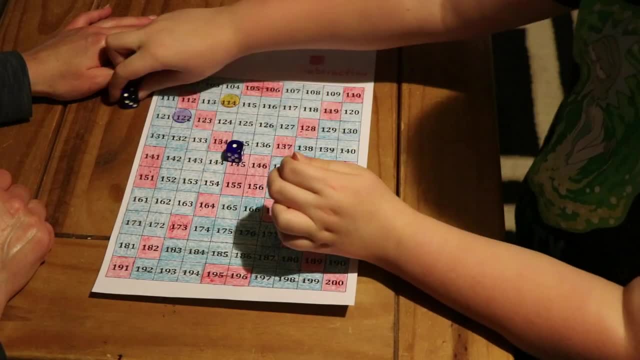 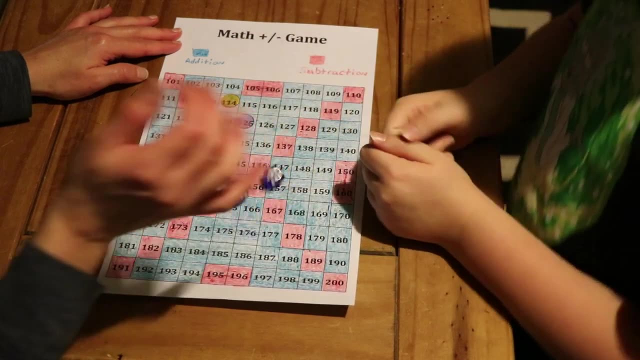 would be subtraction. then he would have gone backwards instead of forward and subtract seven from 115.. Keep taking turns. When it is your turn, roll and move forward or backwards. the total number of squares rolled on the dice. It is okay to land on the same square.